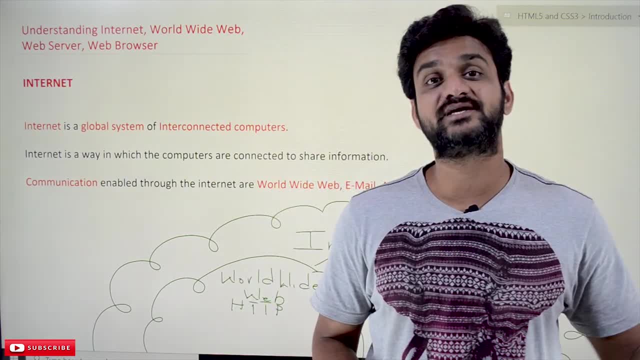 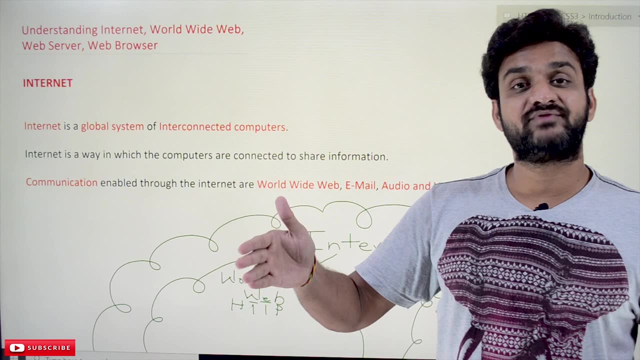 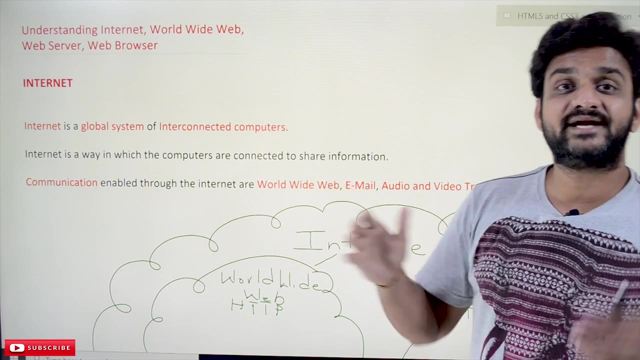 for the playlist is provided in the description below. Now, coming to this class, we will try to have an introduction about internet, old wide web web server and web browser. So this is the terminology which helps us a lot in getting some idea about what happens. what 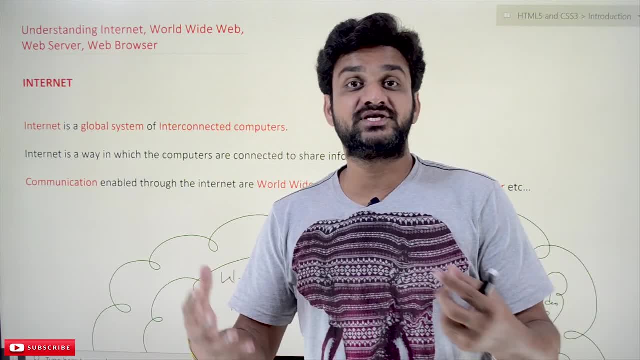 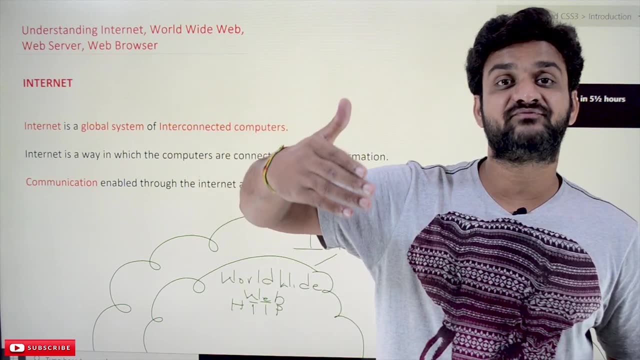 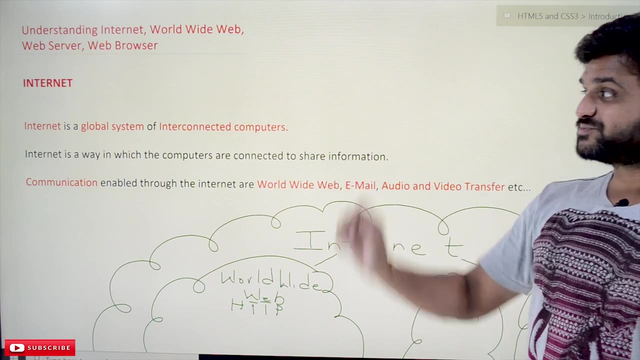 is happening in behind the scenes. So this course is about writing the HTML5 pages and CSS pages in order how the internet, how the world wide web, will work, So that understanding will help us a lot. So, coming to this class, what is meant by an internet? An internet is: a global system of interconnected computers. So I am going to explain what is meant by an internet. An internet is, in one word: an internet is a global system of interconnected computers. So that is the idea of an internet. An internet is a global system of interconnected 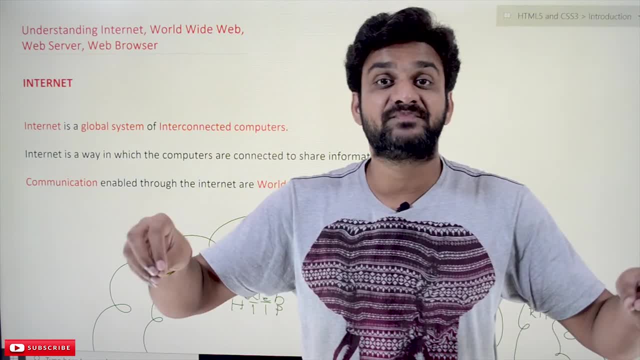 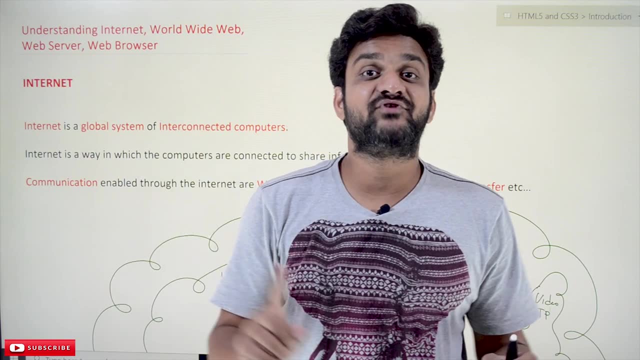 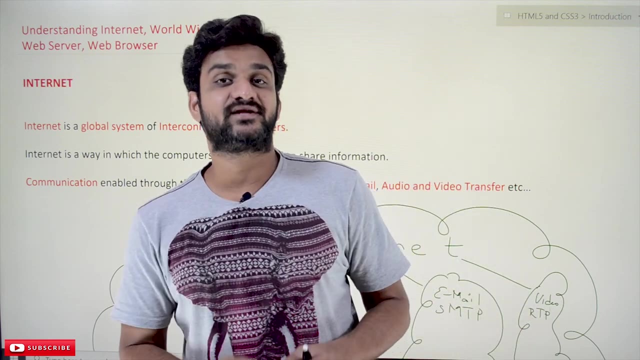 So internet is a global system by which all the computers in this world will get interconnected. So it is a big system where all the systems of this world, of this entire world, will get connected. For example, if you want to get an internet connection, so is it directly available in the computer. 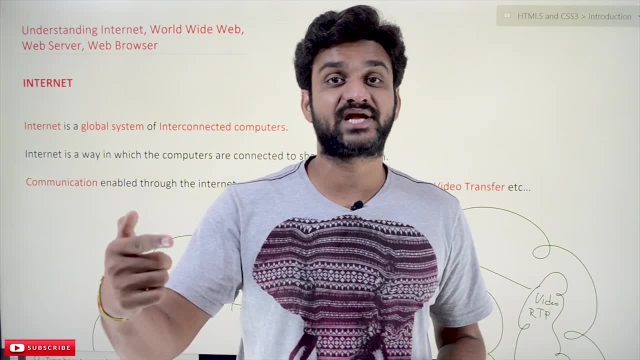 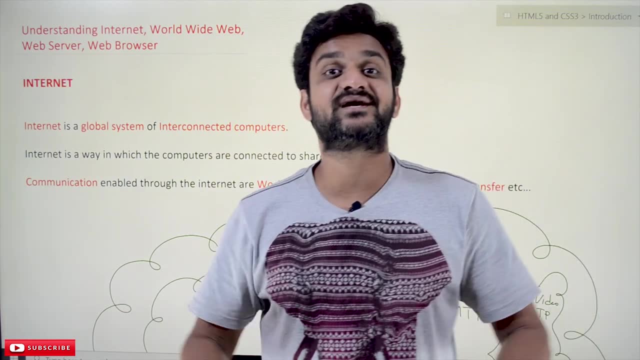 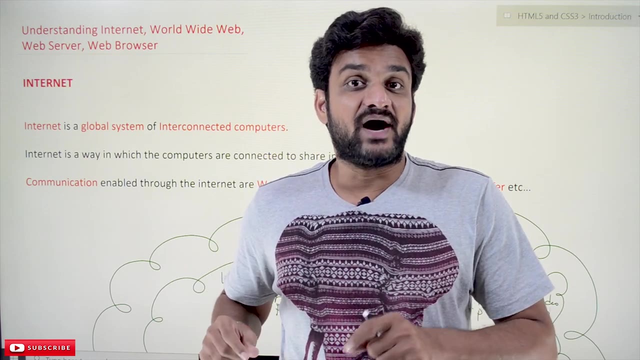 So it is not available. So we have to go to the internet subscriber and ask him for an internet connection. So by getting the internet connection. so getting an internet connection means what? So getting an internet connection means interconnecting our computer to the world. 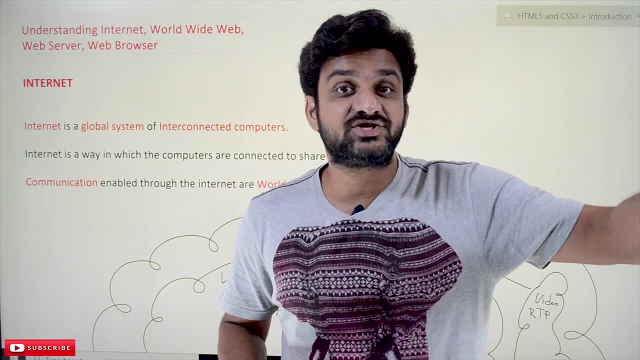 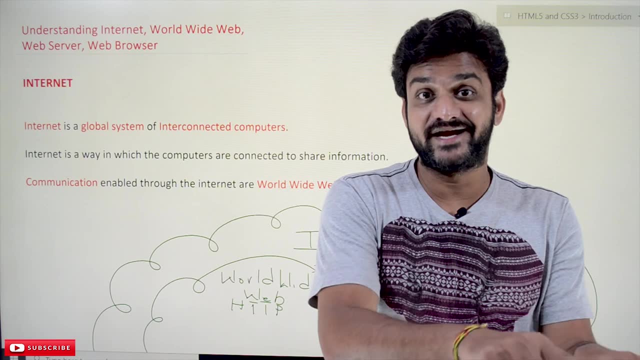 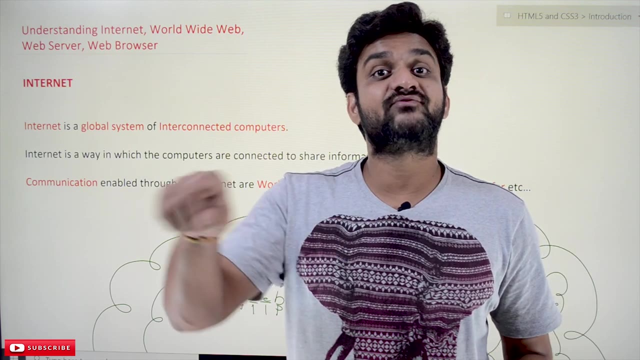 So this world of networks, so this interconnection of the world networks to that world of networks, our computer is also getting connected, So that is what we call it as internet. Internet is nothing, but it is interconnected. So all the networks will get interconnected globally. 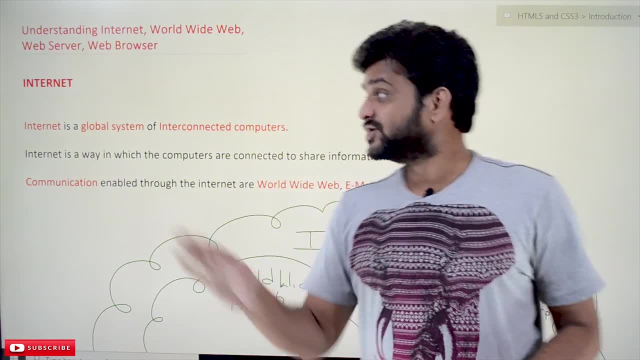 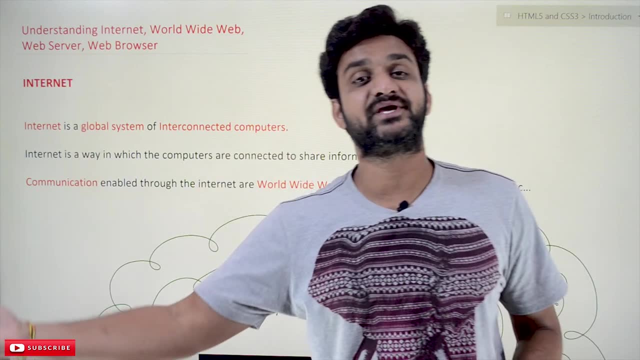 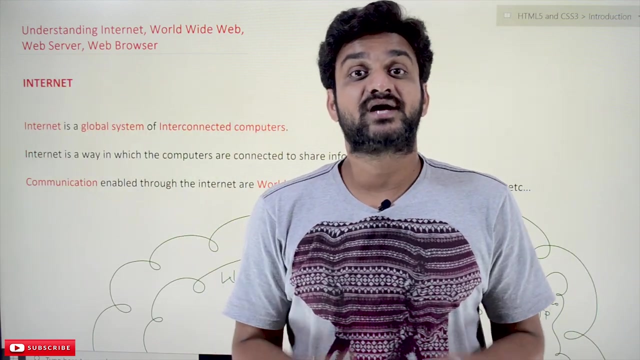 That is what we call it as internet, So this course itself. so understanding about the internet, how the interconnections will happen, how the data is getting communicated from one system to another system. So all these concepts are dealt in a separate course called computer networks. 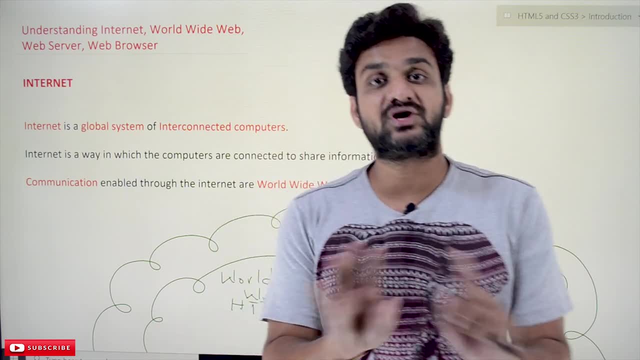 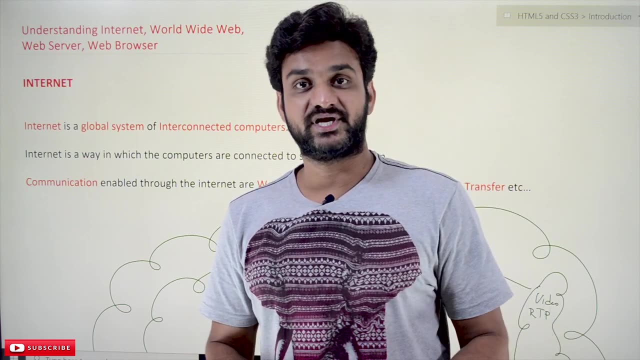 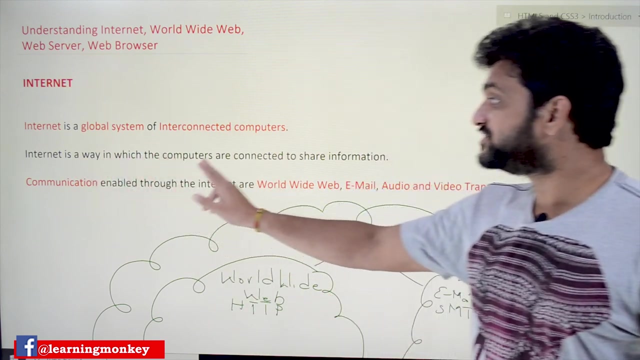 So understanding of computer networks is not required at this point of time. for this course, It is not required to have an understanding about the computer networks. So just to have a brief understanding, we are discussing about these concepts. So internet is a way in which computers are connected to share information. 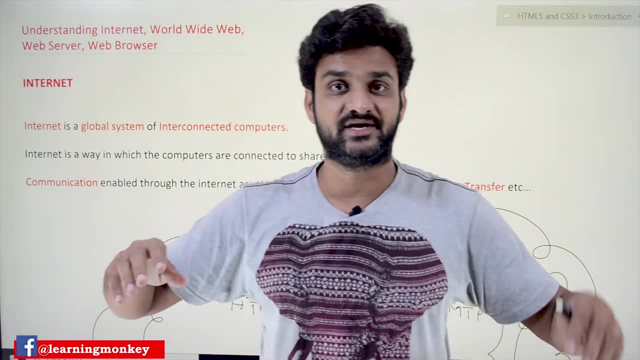 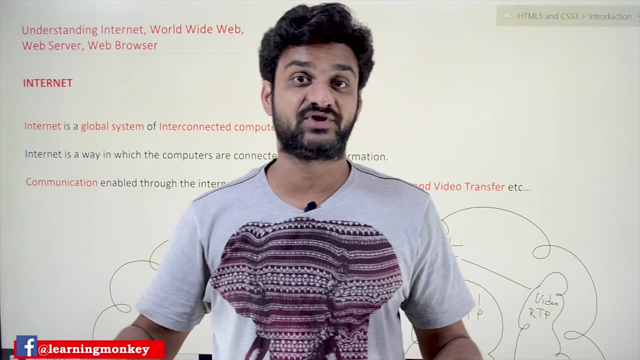 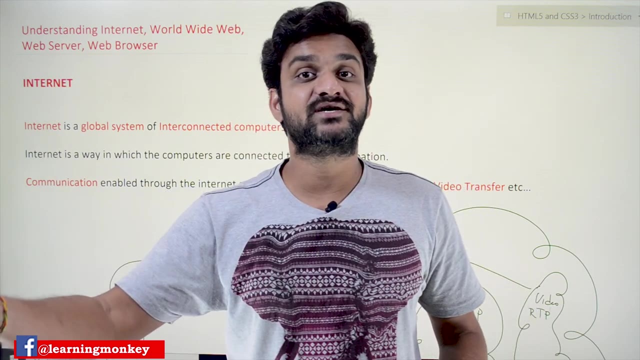 Why these computers are interconnected, Why this global network is being made. So the ultimate objective is to share the information, So the ideas that every person is having will be put on to the internet, And that ideas will be shared among the people who are getting connected to the internet. 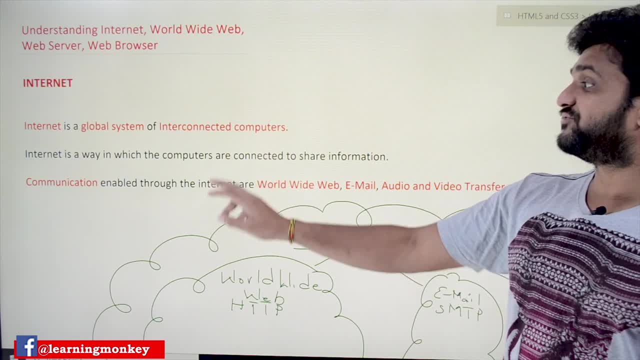 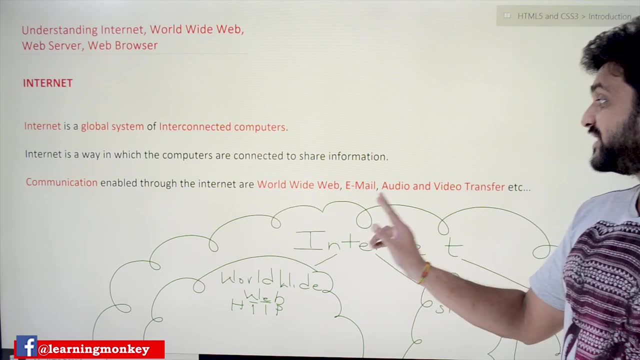 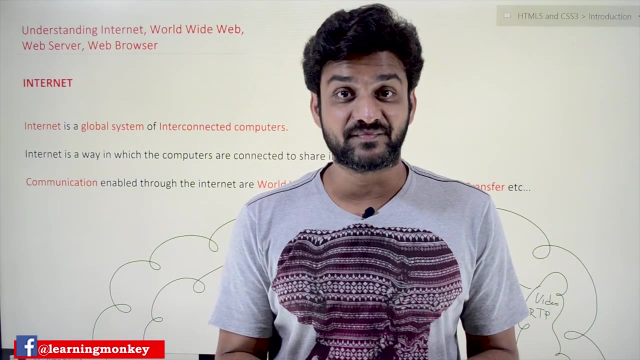 So that is what the objective of an internet, So communication enabled through the internet, are world wide web email, audio and video transfer. So most of the people think that both the internet and world wide web are same. They are not same And most of the people interchangeably uses the internet. 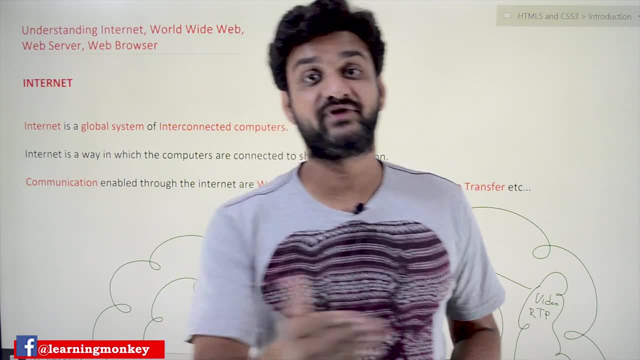 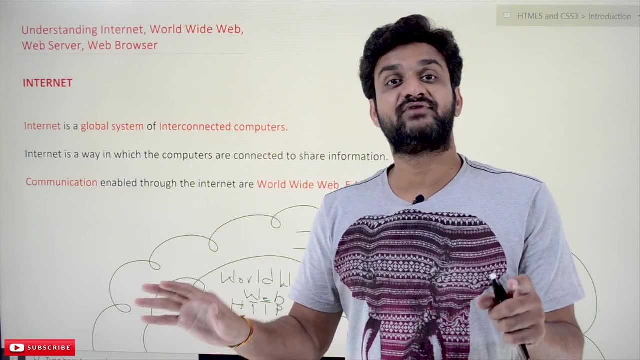 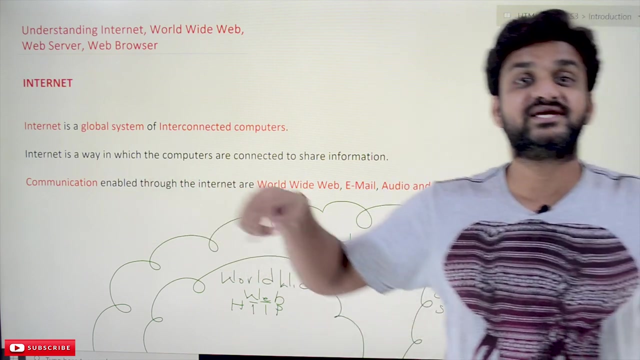 The internet as the world wide web and the world wide web as the internet. Both of them are not same. So what is an world wide web and what is an internet? So the communications that are enabled through the internet. So, within this interconnection of networks, what kind of communications that are enabled are? 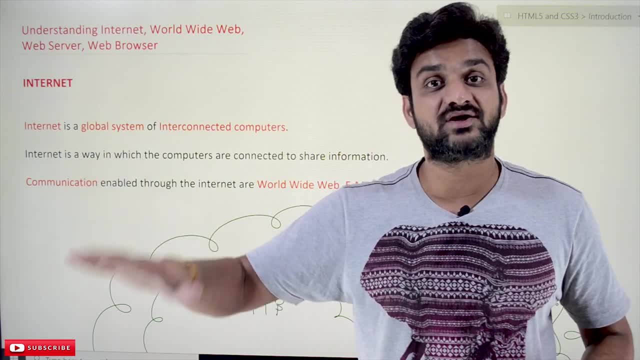 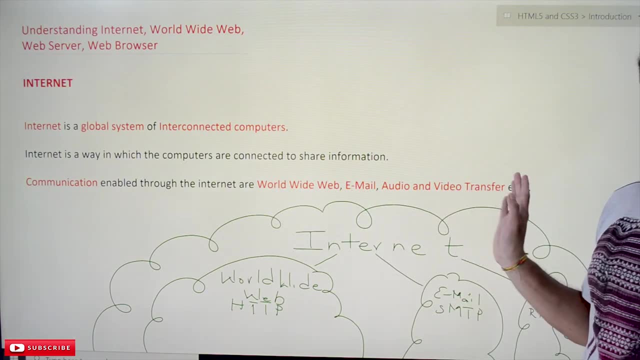 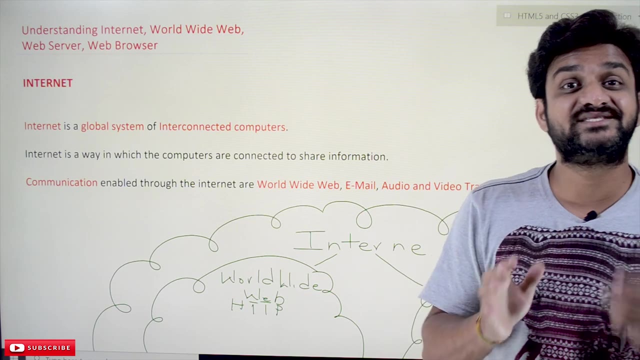 So the communication, the different types of communications that are enabled on the internet are- It is world wide web- email, audio video transfer, etc. So file transfers, hypertext space transfers. So world wide web is just a subsystem of the internet. 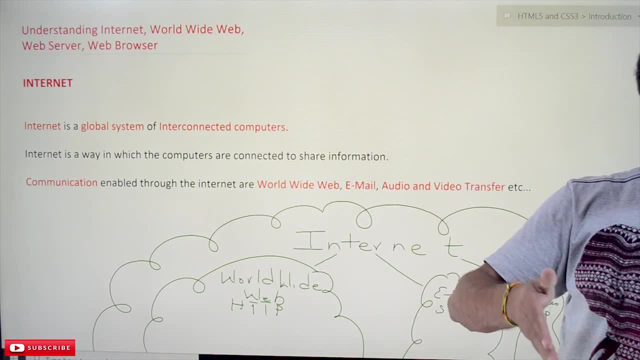 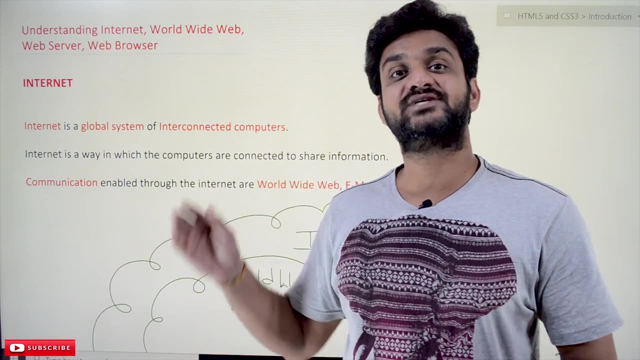 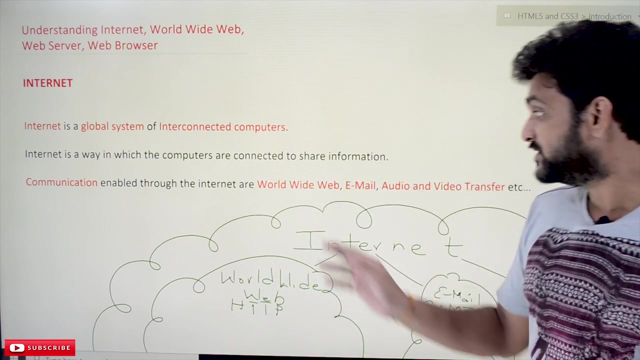 In the same way, email services. So the services that are provided on the internet, The kind of services, the communication that is enabled on the internet is one of them- is world wide web. So that is the difference, The difference between an internet and the world wide web. 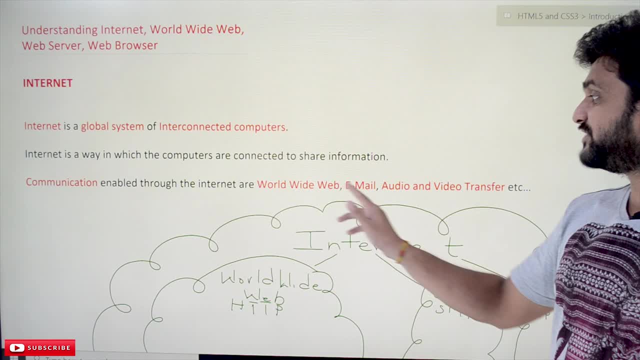 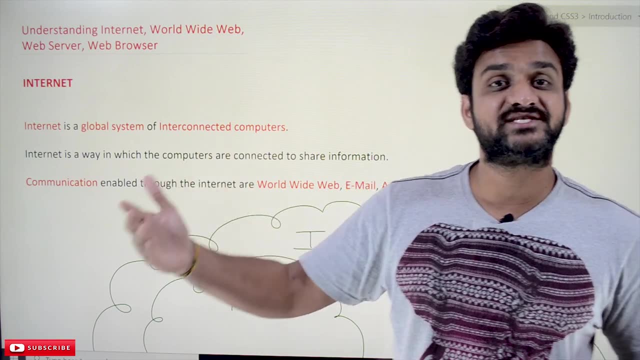 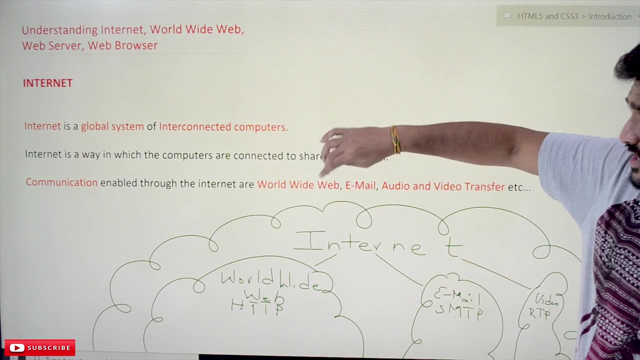 So one of the services, the communications enabled through the internet or world wide web, Email, audio video services like YouTube, email services like Gmail, These are the kind of communications that are available, that can be enabled on the internet. So now to have the visualization of internet and world wide web. 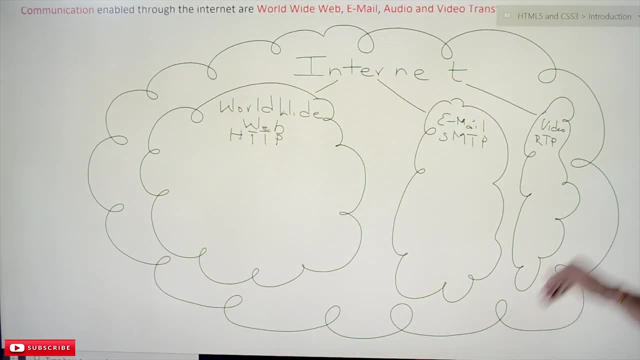 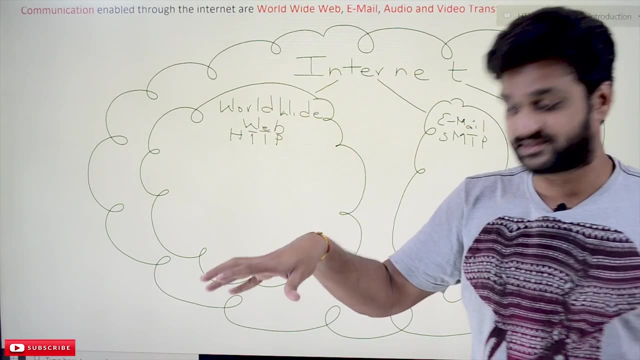 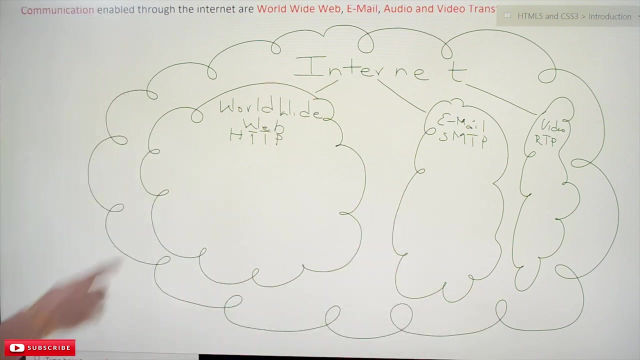 Let's see this. So this bigger circle is what we call it as An internet. Within that internet, the kind of communications that are possible, The services. So, in short, to understand better, the services that can be enabled on the internet are- It is world wide web, email and video audio transfer. 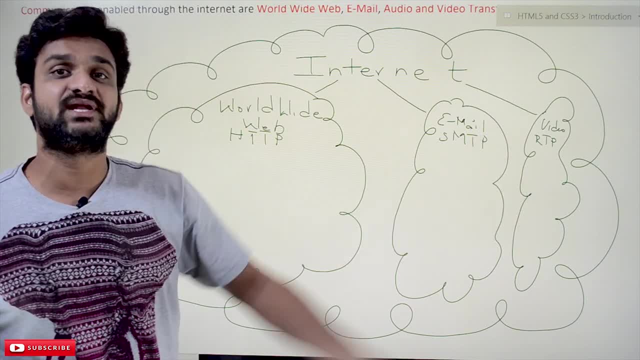 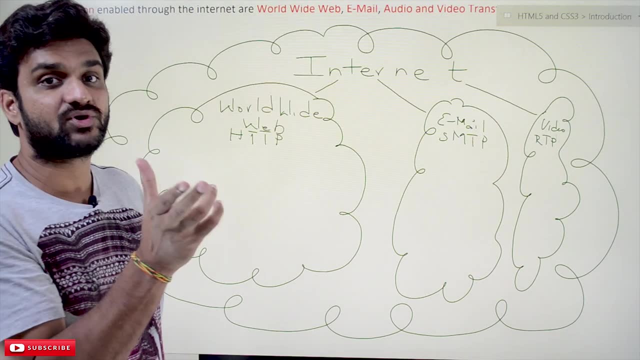 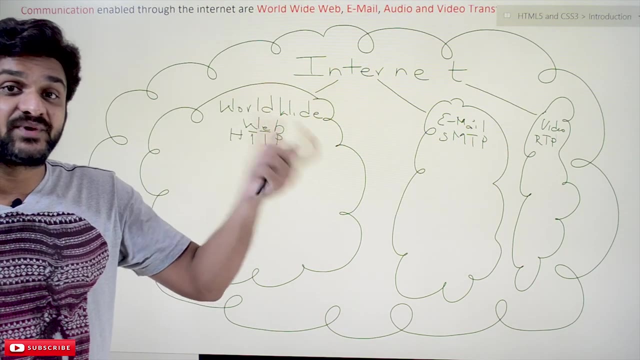 And there are many other kind of services that are available. So these are some of the services. So these services are provided by certain kind of protocols called HTTP. So world wide web means the web pages, The hypertext, can be transferred from one system to another system. 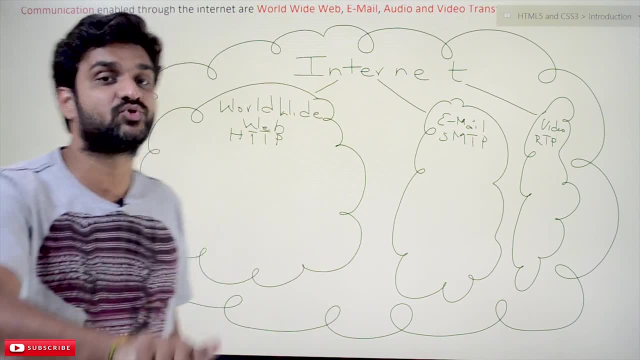 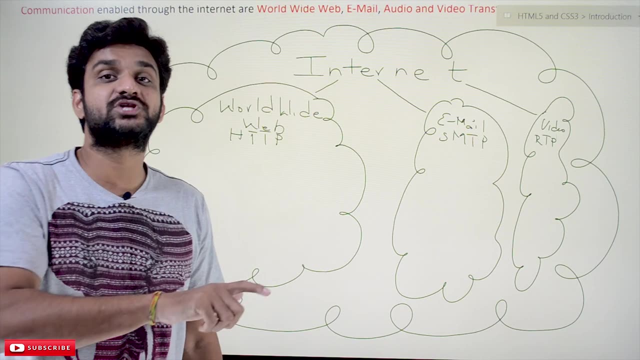 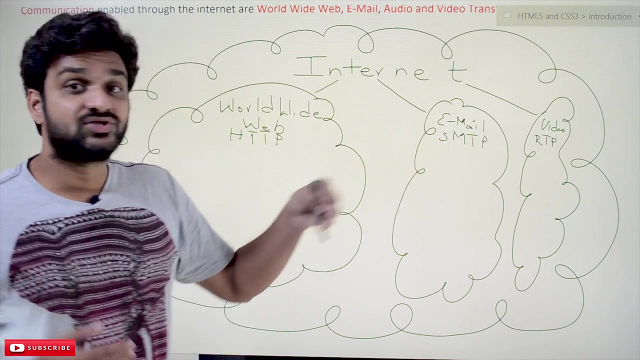 Within the internet is done by the protocol called HTTP. HTTP stands for hypertext transfer protocol, So based upon that protocol, the web pages can be transferred from one system to another system. Similarly SMTP, So the mailing services that are provided on the internet. 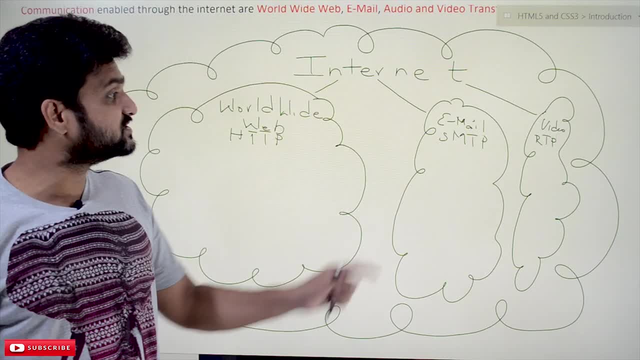 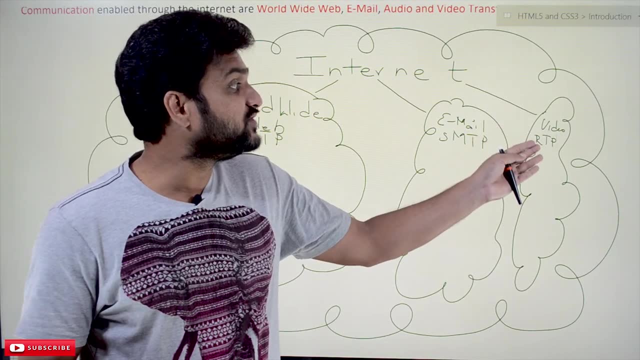 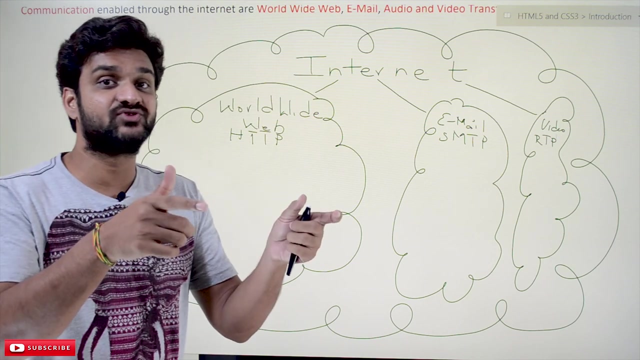 Can be transferred from one system to another system By using a protocol called SMTP, Simple mail transfer protocol. For audio and video services, it is RTP, Real time transfer protocol. So what is the differentiation that you can make between the internet and the world wide web is? 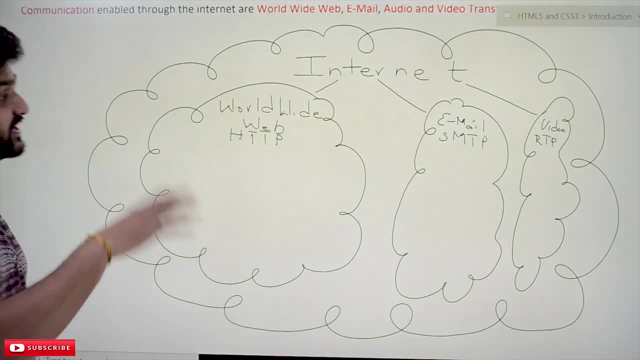 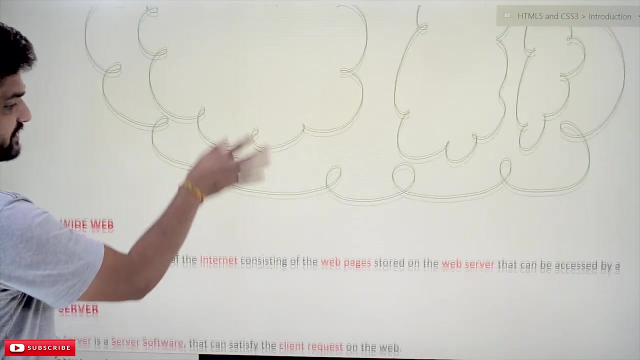 Internet as a whole provides some services called world wide web email and RTP. So world wide web is a system, It is a subsystem of internet. So let's try to understand the definition of the world wide web. So what is this world wide web is? 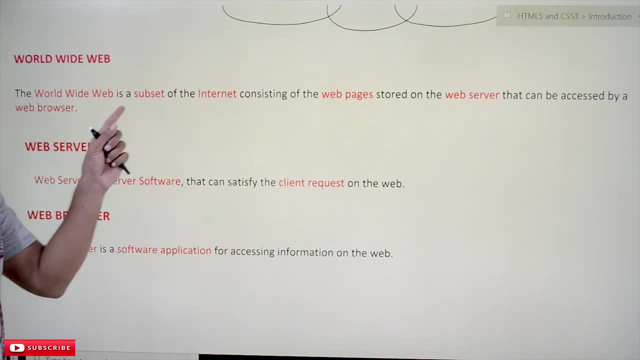 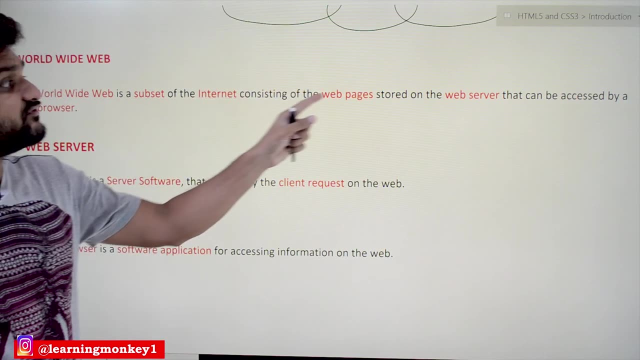 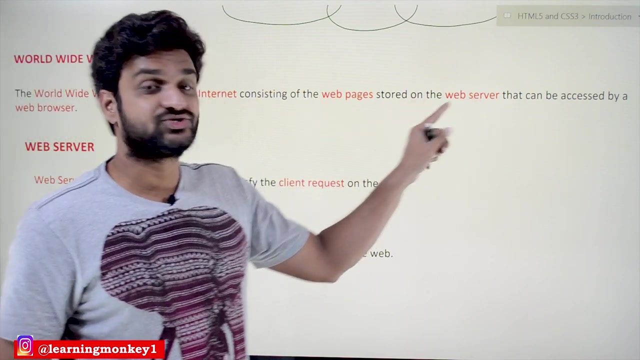 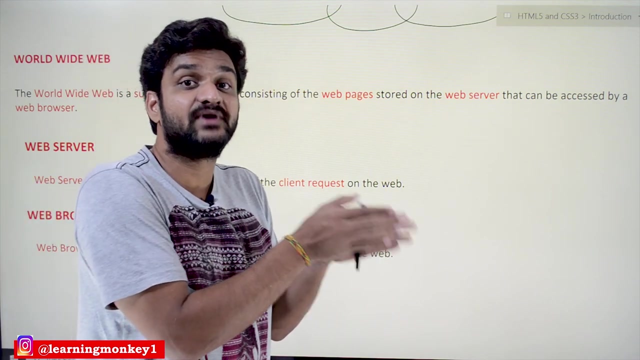 The world wide web is a subset of internet, As we have seen in our diagram. it is just a subset of internet consisting of web pages. So this entire world wide web consists of web pages stored on a machine, So stored on web server. So these web pages are stored on a machine called web server. 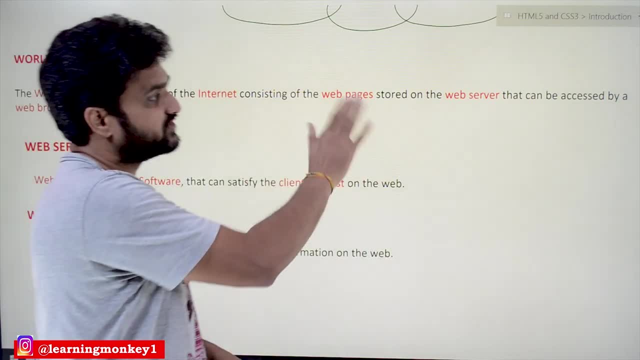 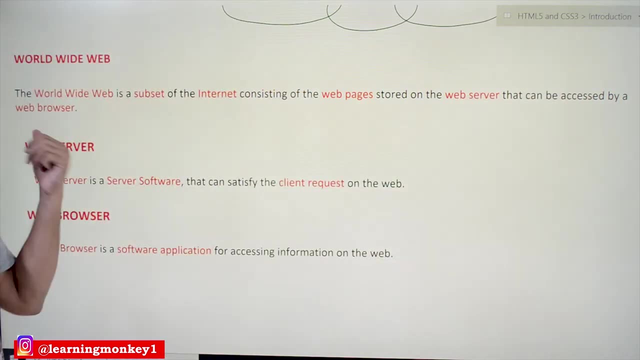 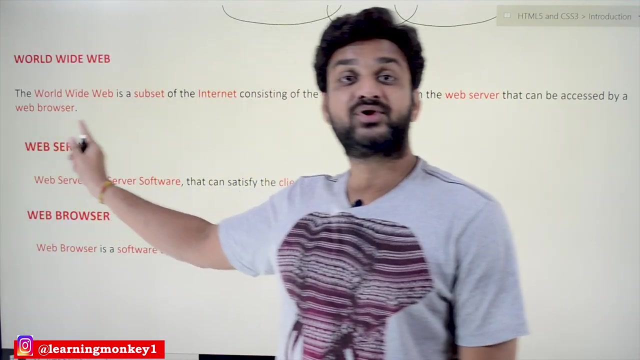 Or a software called web server. So what is that web server? that we will try to understand. So these web pages are stored on web server That can be accessed by web browser. So the pages which are stored on the web server Can be accessed by the web browser. 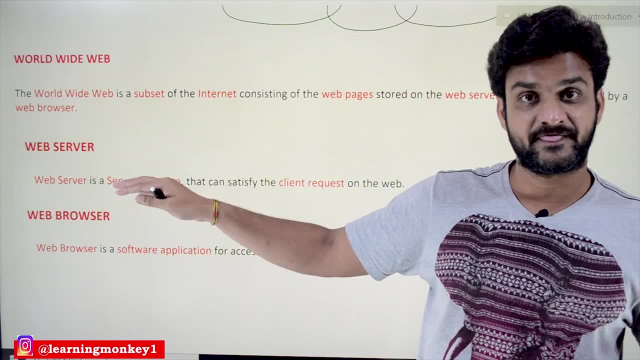 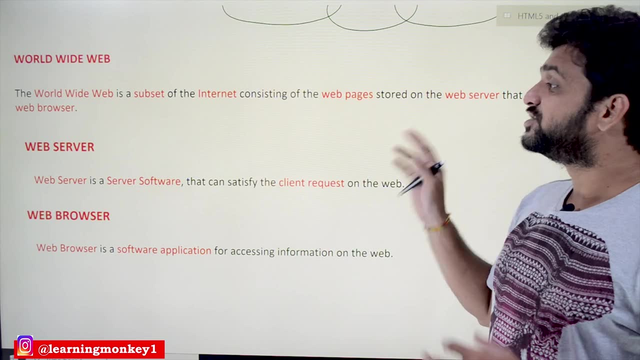 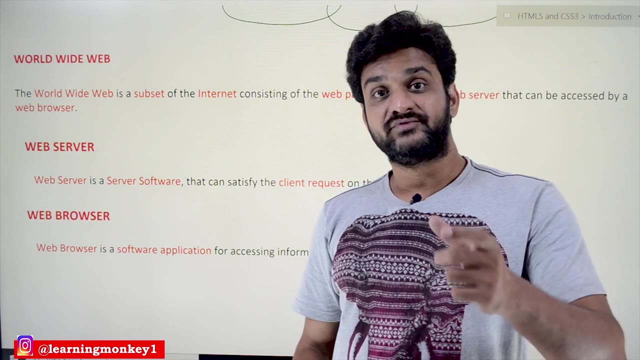 So this is what we call it as old wide web. Now, what is meant by web server? As we have said that the web pages are stored on web server. So what is meant by web server? Web server is a server software. It is a software which is stored on a hardware. 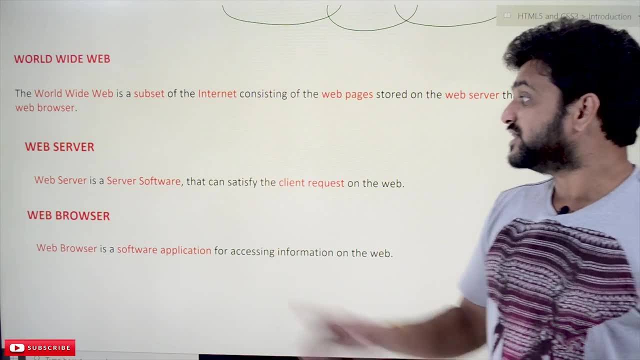 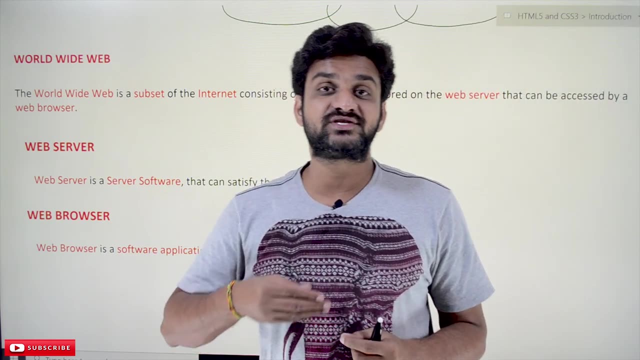 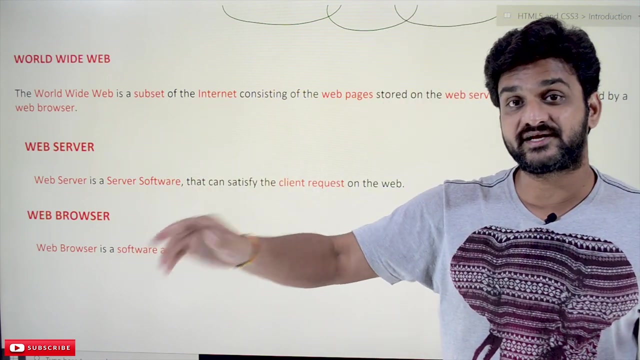 So that entire machine is what we call it as a server That can satisfy the client request on the web. The user who is trying to access the information on the internet Is what we call it as users of the internet, Which is done by an application called client. 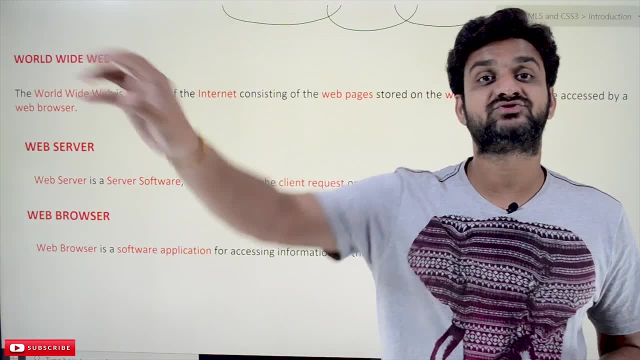 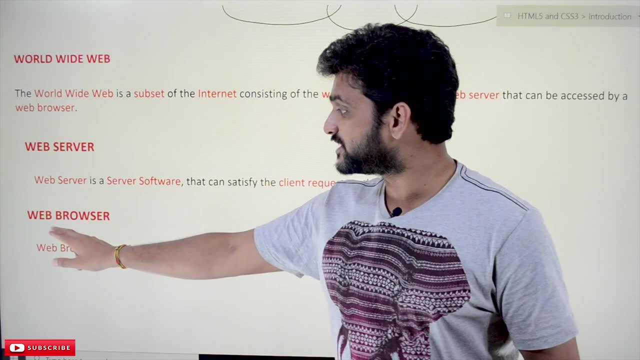 So the user who is accessing the resources on the web Is what we call it as, whom we call it as a client. So what that client is Is what we call it as web browser. Web browser is a software application for accessing information on the web. 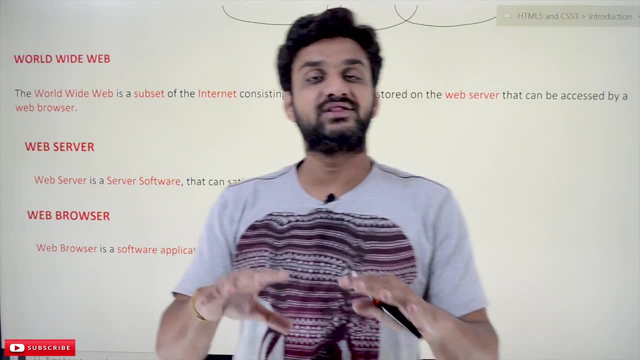 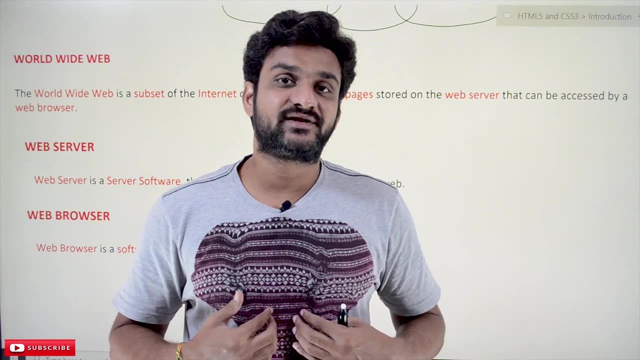 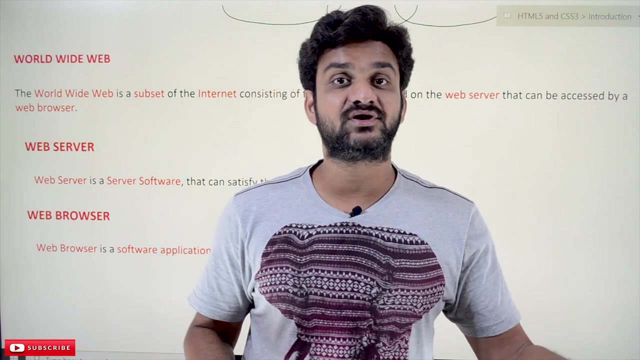 So, to elaborate these all these things in a single explanation, What we will do is So, once we want to take the internet connection, So, after getting the internet connection, What we are capable of. So, without internet connection and with internet connection, What is the difference? 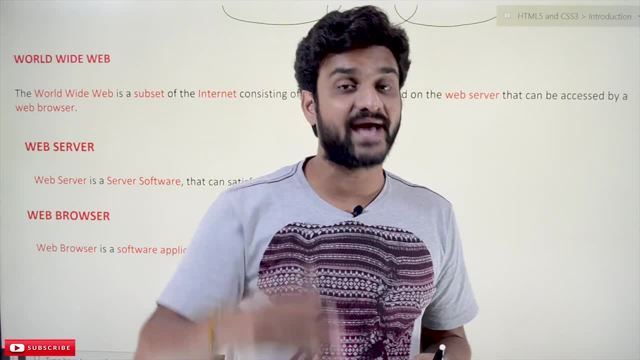 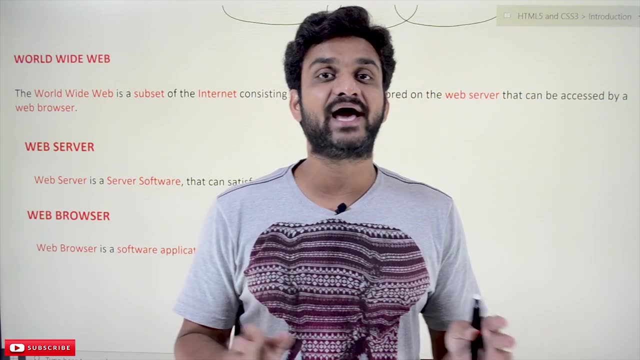 With the internet. without internet connection, Is it possible for you to access Google? Is it possible for you to access Facebook? No, this is not possible for you to access Facebook, Google, Gmail And YouTube is not possible. You can access without the internet connection. 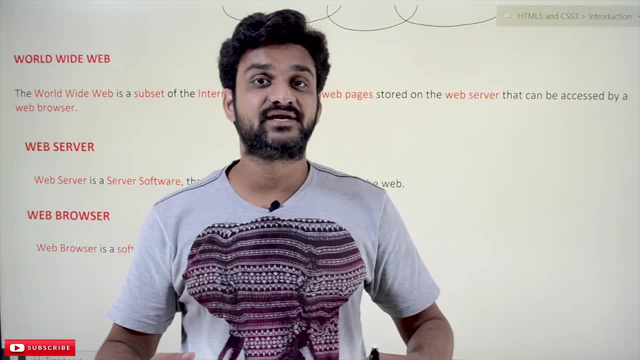 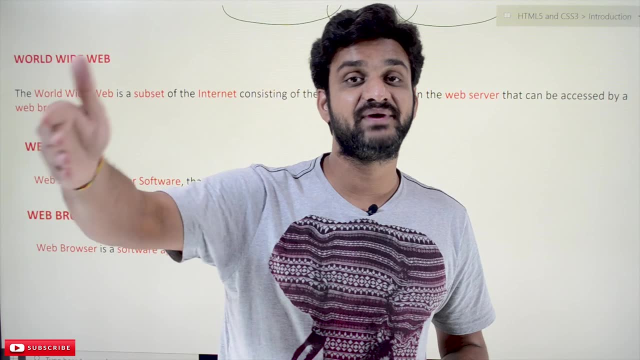 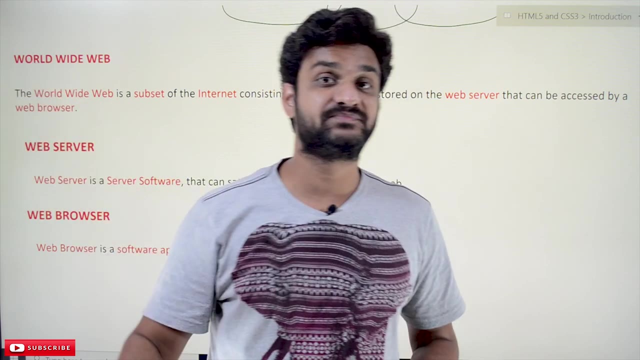 So after getting the internet connection, After getting the internet connection, We can access the stuff which is stored on the web servers Like Google, Gmail, Email, So Gmail, YouTube and all those. We can access the content which is stored on those web servers. 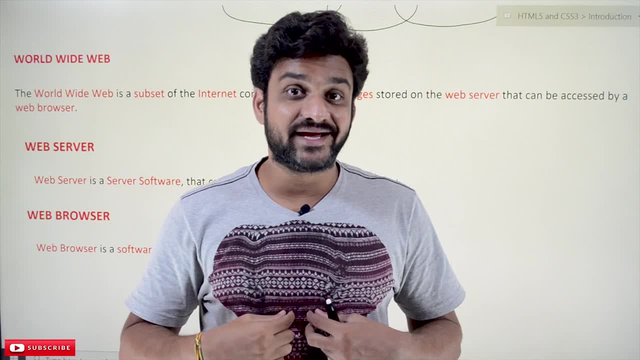 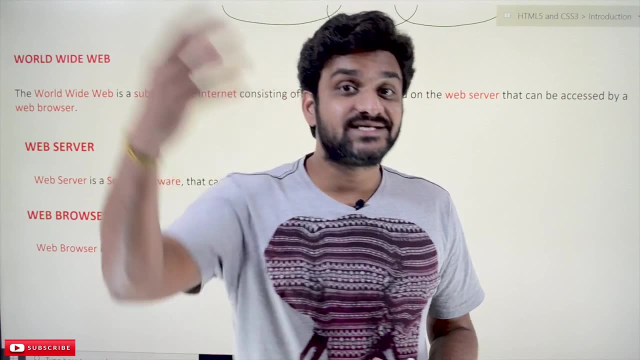 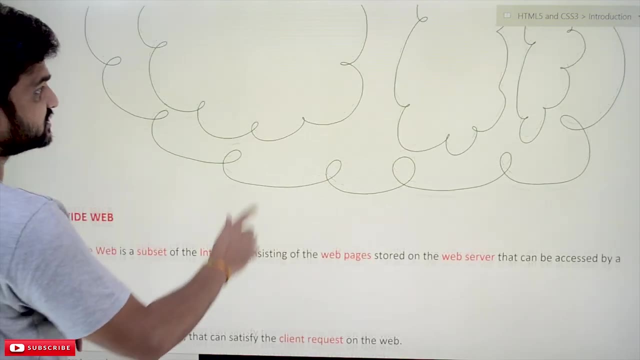 So, with the internet connection, Being the clients of the internet connection, Users of the internet connection, We can access the information that is stored on the web server. So let's try to visualize this within this diagram. So what happens with the internet connection is: 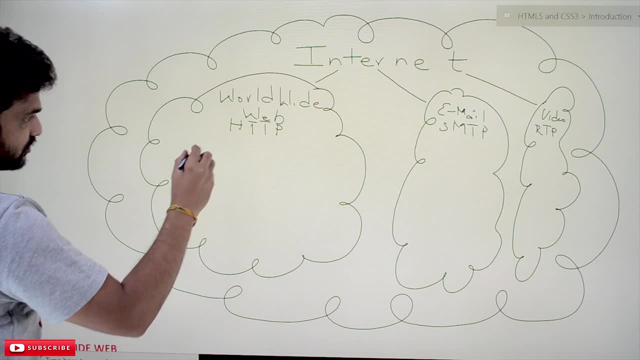 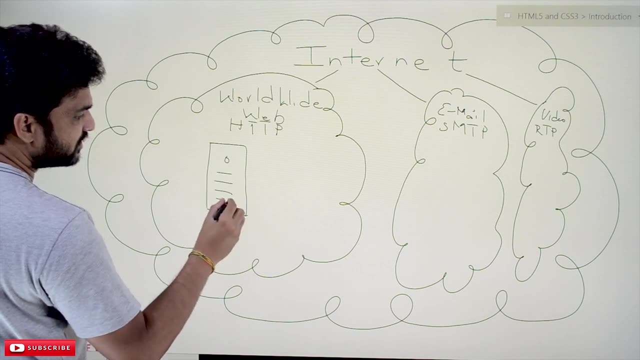 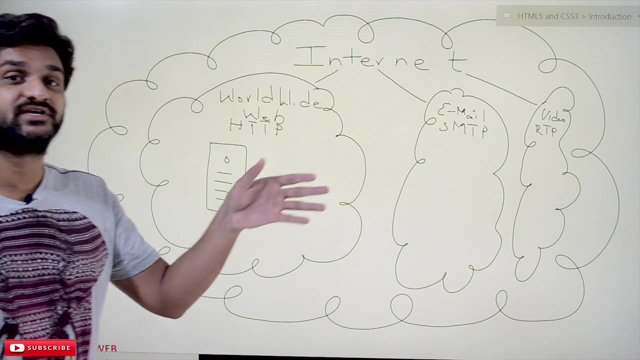 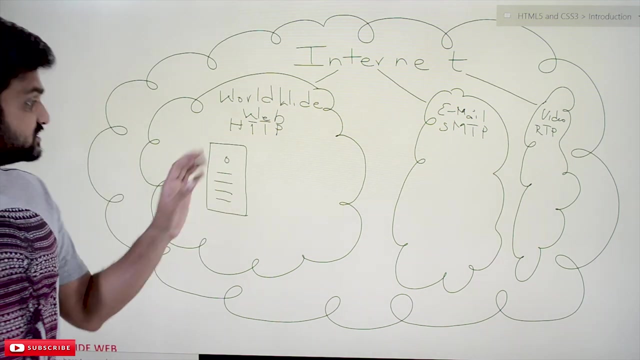 So this is what we call it as web server: Nothing but a system Within which we have that server software. So what that server software is capable of is, It is capable of So on this server. So, for example, if you consider this as a Facebook server, 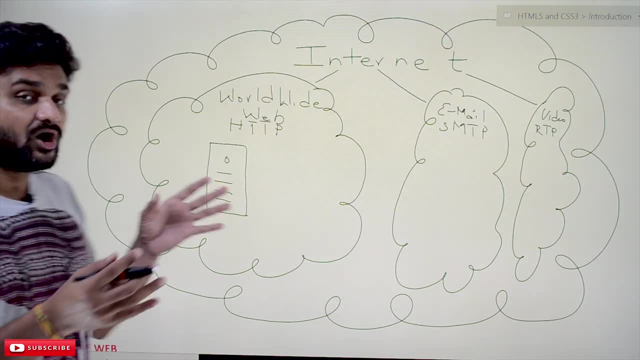 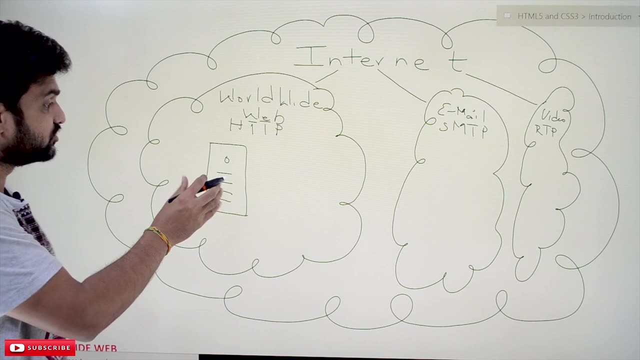 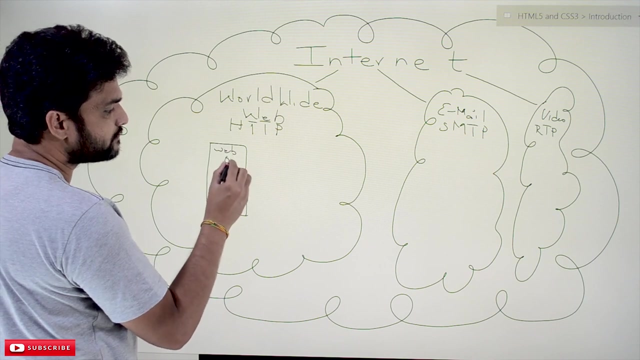 Consider this as a Facebook server, So all the pages which are related to the Facebook will be stored on this server. Okay, So all the pages- Web pages- will be stored on this. Web pages will be stored on this server. So, being the client. 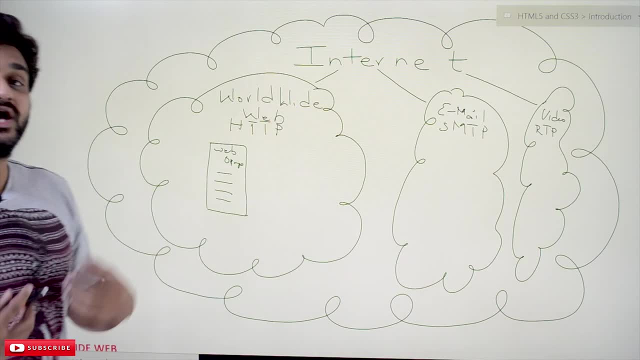 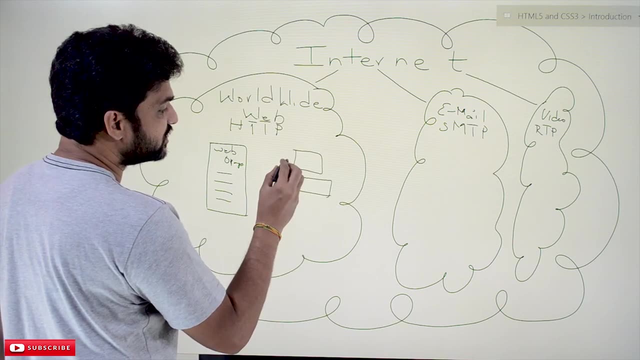 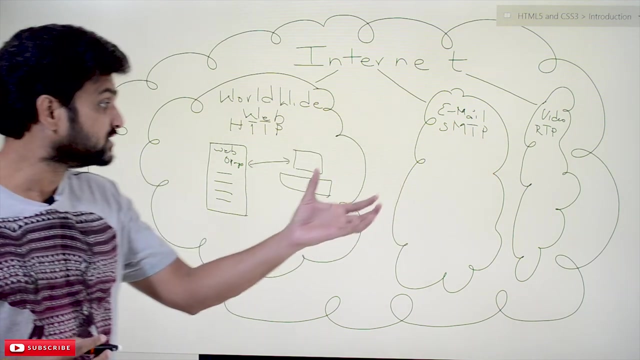 Being the user of the internet. So now I have taken the internet connection, Now I am the user of the internet connection, So I am what we call it as a Myself is called as a client. So what is the application which is making? 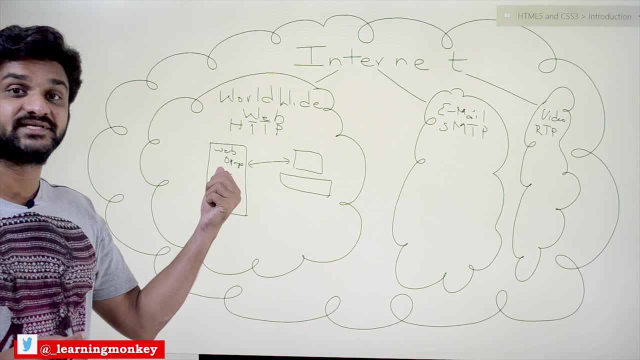 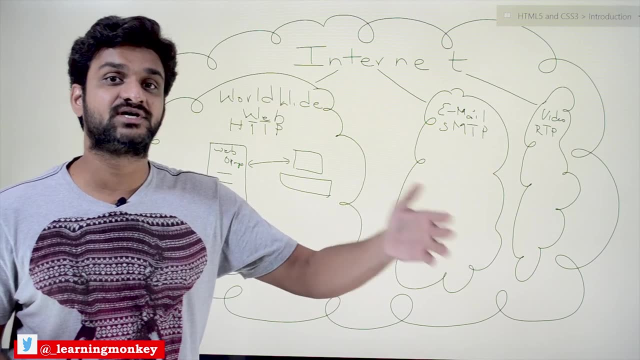 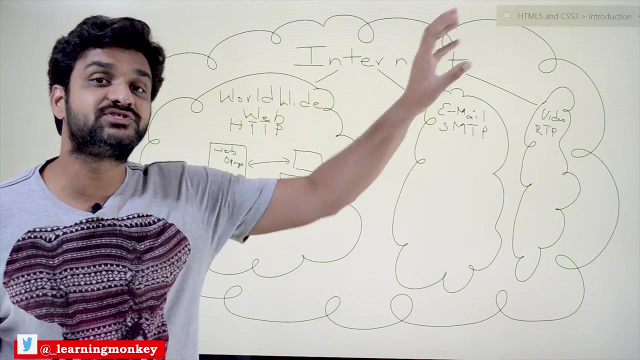 Making us to access the content on these web pages. Content of these web pages is what we call it as a browser. So Google Chrome, Mozilla Firefox, Safari, So all these are the applications Which are capable of accessing the web pages which are stored on the internet. 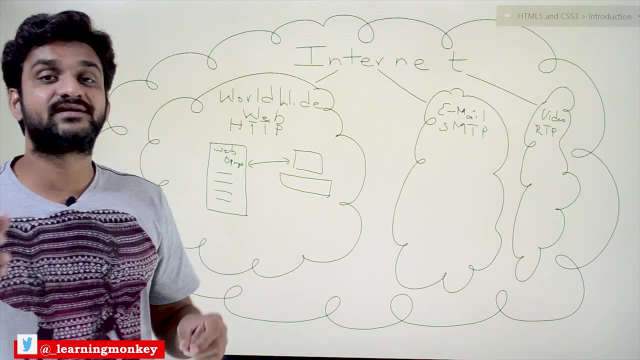 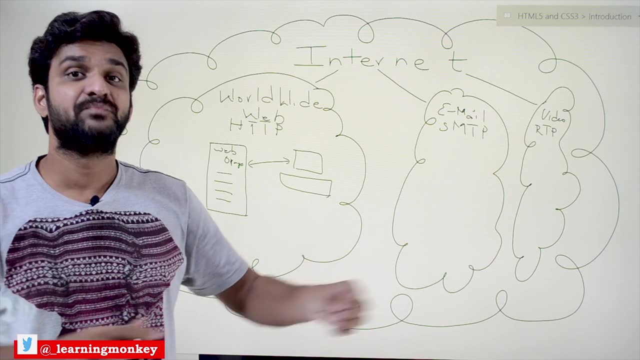 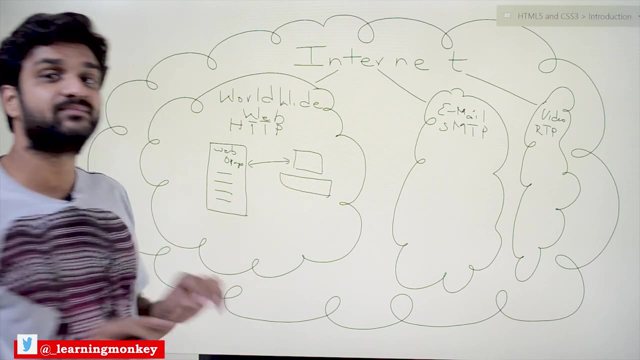 On the web servers. So it will, It will get, It will go to those web servers. So there are different types of web servers. So, where the applications are stored, Millions of millions of web servers where the applications are stored. So, while typing here, wwwfacebookcom. 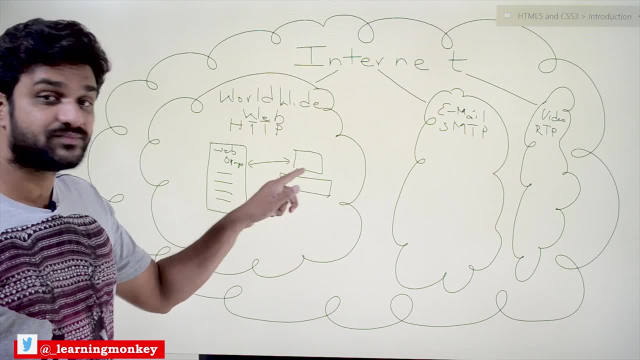 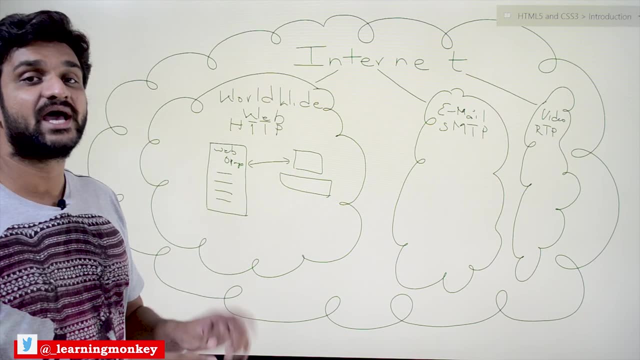 What happens is, This is what we call it as a browser. In the browser, we will type wwwfacebookcom, Right. So, after typing it and entering it, What happens is This browser is capable of So within which, Within this, we are having different kinds of systems. 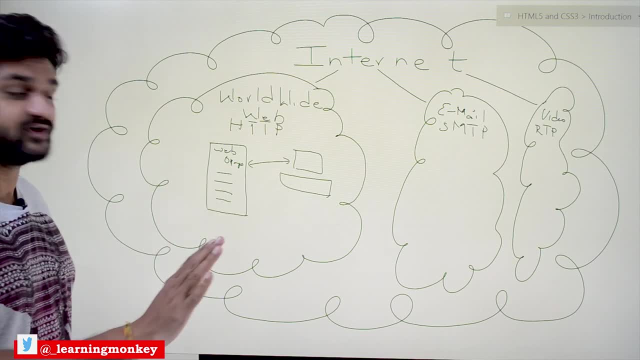 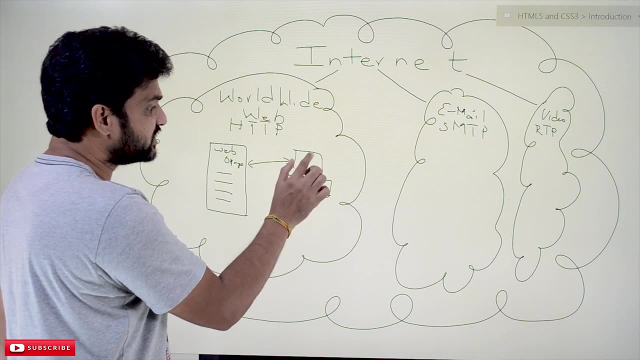 So it itself is a separate course called computer networks. Let's try to understand in a simpler way That this is what we call it as a client. This client will access these web pages, So it is a Facebook server, FB server, So it is going to this FB server.